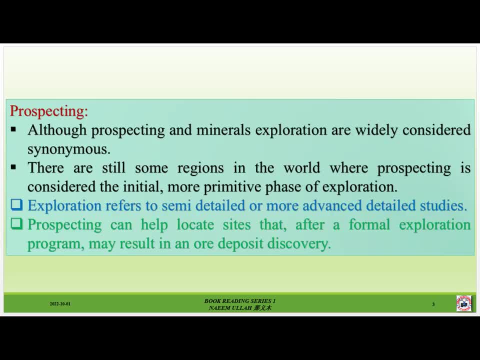 understanding the genesis of our deposits. Prospecting: Although prospecting and minerals exploration are widely considered synonymous, there are still some regions in the world where prospecting is considered the initial, more primitive phase of exploration. Exploration refers to semi-detailed or more advanced detailed studies. Prospecting can help locate. 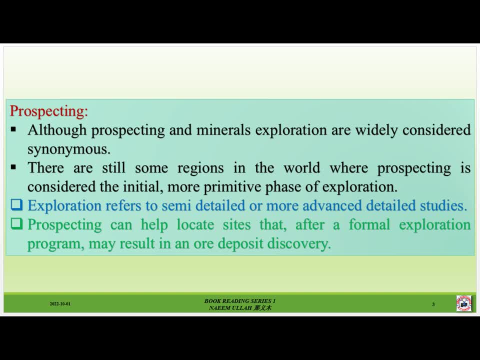 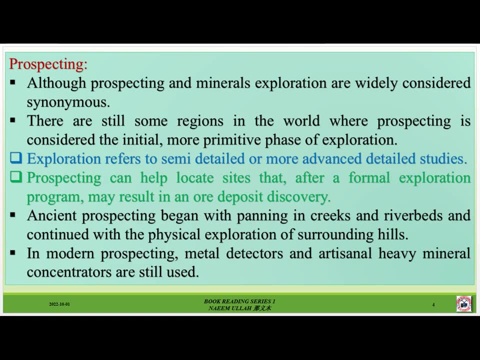 sites that, after a former exploration program, may result in an ore deposit discovery. Although prospecting and minerals exploration are widely considered synonymous, there are still some regions in the world where prospecting is considered the initial, more primitive phase of exploration. Exploration refers to semi-detailed or more advanced detailed studies. Prospecting can 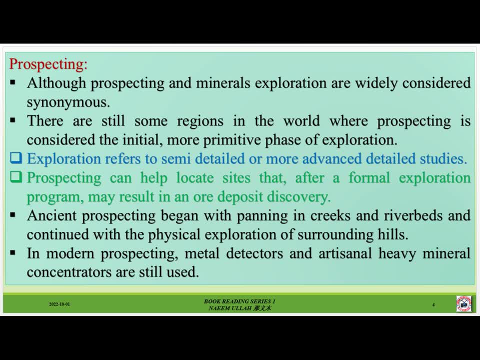 help locate sites that, after a former exploration program, may result in an ore deposit discovery. Ancient prospecting began with panning in creeks and riverbeds and continued with the physical exploration of surrounding hills. In modern prospecting, metal detectors and 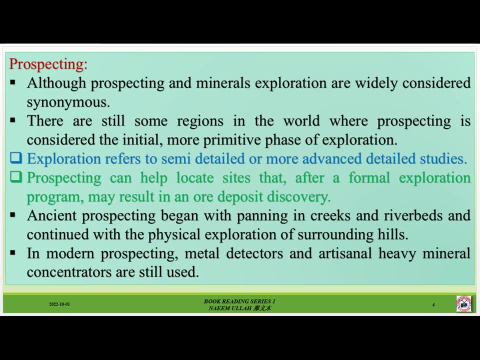 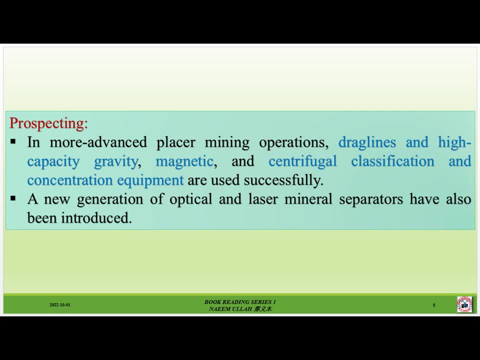 artisanal heavy mineral concentrators are still used In more advanced placer mining operations. dragon lines and high-capacity gravity magnetic and centrifugal classification and concentration equipment are used successfully. A new generation of optical and laser mineral operators have also been introduced. 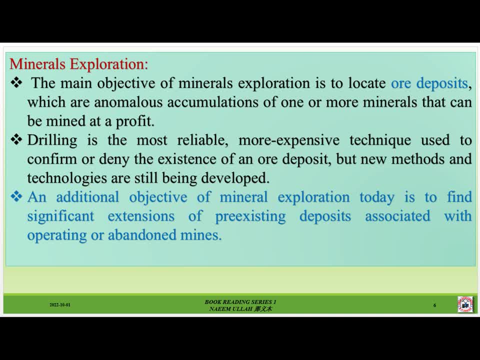 Exploration can help locate sites that, after a former exploration program, may result in an ore deposit discovery. Minerals Exploration. The main objective of minerals exploration is to locate ore deposits, which are anomalous accumulations of one or more minerals that can be mined at a profit. 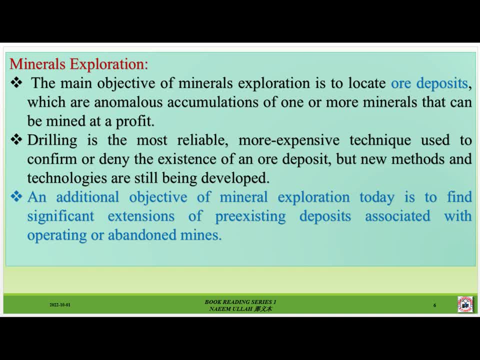 Drilling is the most reliable, more expensive technique used to confirm or deny the existence of an ore deposit, but new methods and technologies are still being developed. There are one iron work at a time: Actionا. The operational objective of mineral exploration today is to find significant extensions of 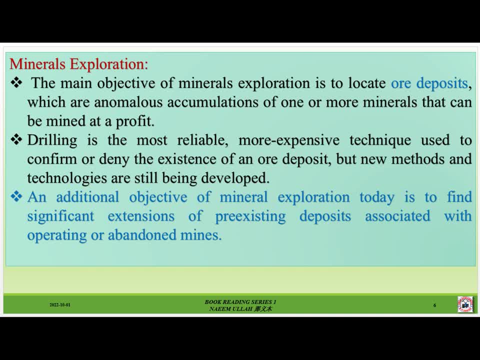 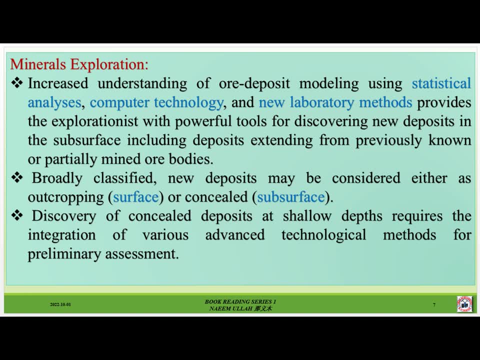 pre-existing deposits associated with operating or abandoned mines. Increased understanding of ore deposit modeling using statistical analysis, computer technology and new laboratory methods provides the explorationists with powerful tools for discovering new deposits in the subsurface, including deposits extending from previously known or partially mined ore. 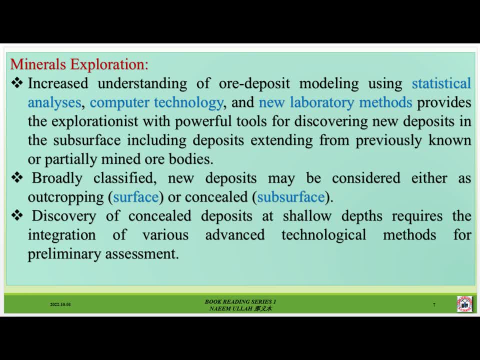 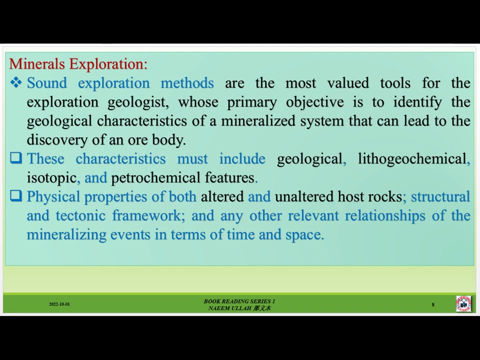 bodies Broadly classified. new deposits may be considered either as outcropping surface or concealed subsurface. Discovery of concealed deposits at shallow depths requires the integration of various advanced technological methods For primary assessment. sound exploration methods are the most valued tools for the geological characteristics. 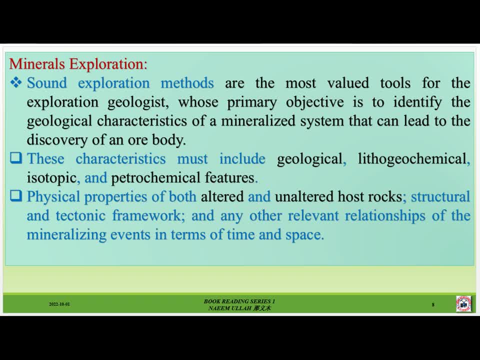 Exploration geologists whose primary objective is to identify the geological characteristics of a mineralized system that can lead to the discovery of an ore body. These characteristics must include geological, lithogeochemical, geosynthetic and geological characteristics. P checked. 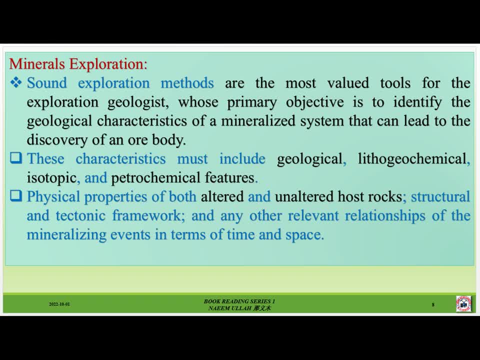 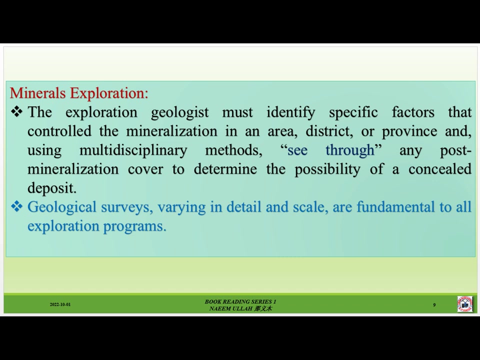 Isotopic and petrochemical features, Physical properties of both altered and unaltered host rocks, Structural and tectonic framework And any other relevant relationships of mineralising event in terms of time and space. The exploration geologists must identify specific factors that control the mineralisation in. 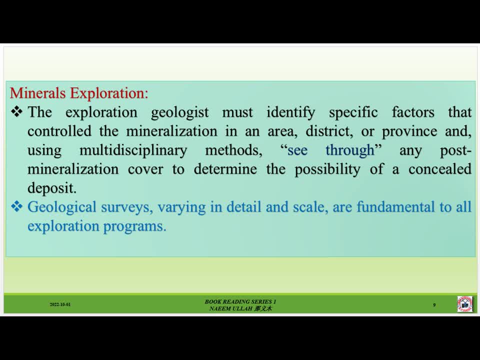 an area, district or province. Treatment of Yoz lava or top參ioc��ts and, using multidisciplinary methods, see through any post mineralization cover to determine the possibility of a concealed deposit. geological surveys, wearing in detail and scale are fundamental to all exploration programs. geological. 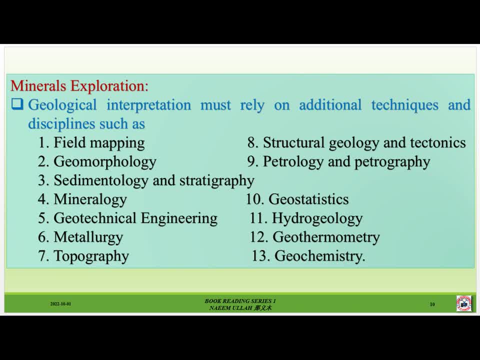 interpretation must rely on additional techniques and disciplines, such as field mapping, geomorphology, sediment ology and a stratigraphy, mineralogy, geotechnical engineering, metallurgy, topography, structural geology and tectonics, petrology and a petrography, geostatics, hydrogeology, geothermometry. 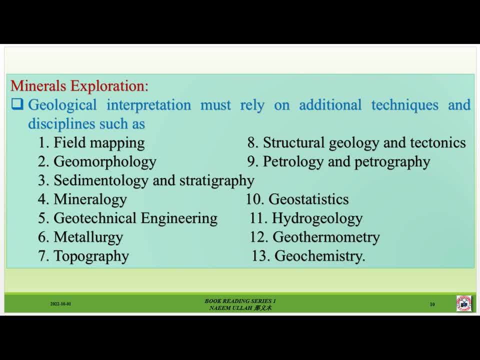 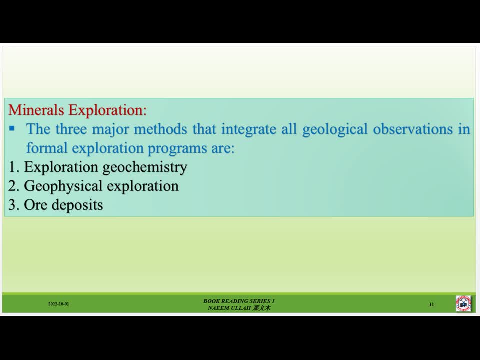 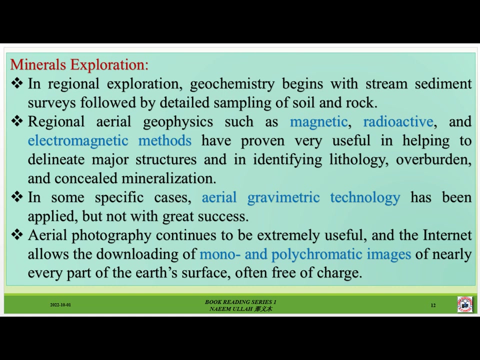 and geochemistry. the three major methods that integrate all geological observations in former exploration programs are: number one, exploration geochemistry. number two, geophysical exploration. number three, or deposits in regional exploration geochemistry begins with stream sediment surveys followed by detailed sampling of soil and rock regional area for geophysics, such as 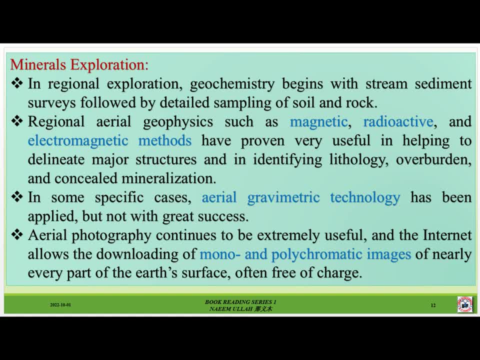 magnetic, radioactive and electromagnetic methods have proven very useful in helping to delineate major structures and in identifying lithology or burden and concealed mineralization. in some specific cases, area gravimetric technology has been applied, but not with great success. area photographic continues to be extremely useful and the 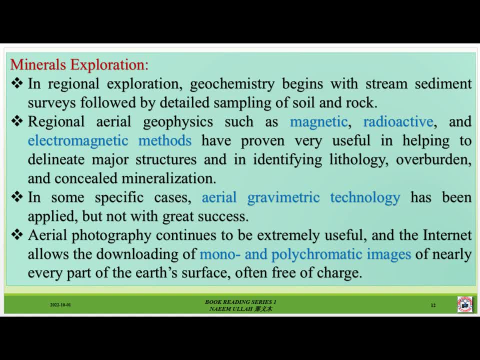 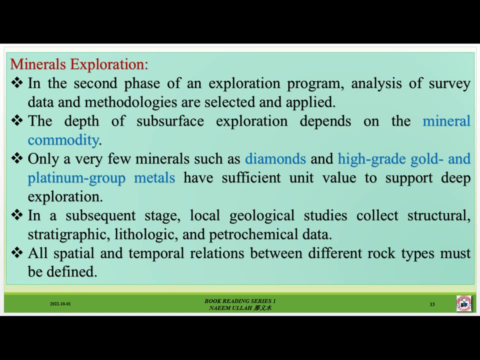 internet allows the downloading of mono and poly chromatic images of nearly every part of the earth's surface, often free of charge. in the second phase of an exploration program, analysis of survey data and methodologies are selected and applied. the depth of subsurface exploration depends on the mineral commodity. only a very few minerals, such 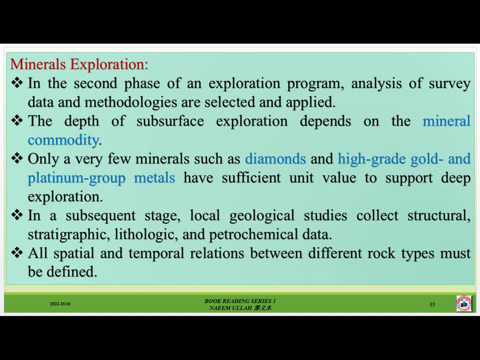 as diamonds and a high-grade gold and platinum group metals, have sufficient unit value him to support deep exploration in a subsequent stage. local geological studies collect structure and stratigraphic lake ology and a petrochemical data. all spatial and temporal relations between different rock types must be defined here. special. 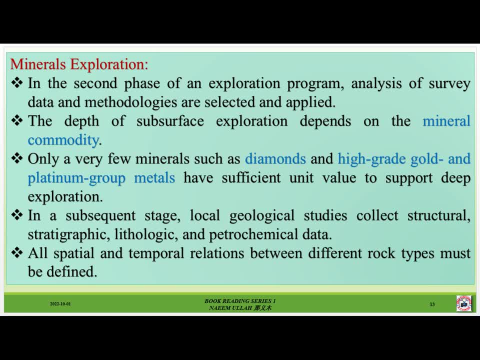 means involving or having the nature of space, is called the spacial map. so when we Philippa stone, a difference between rock types often used to describe the surrounding place, would be returned to ISS Per b, yes, we could have ore system, gemstone navellum doing team crystalCRIES that argue differentHOE aquele. 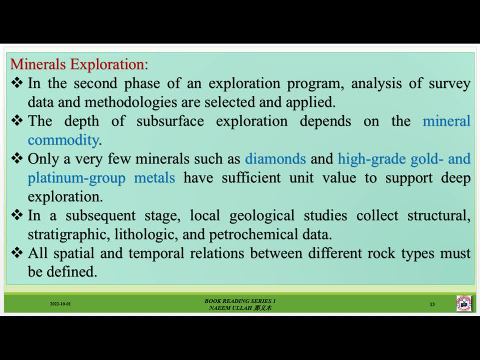 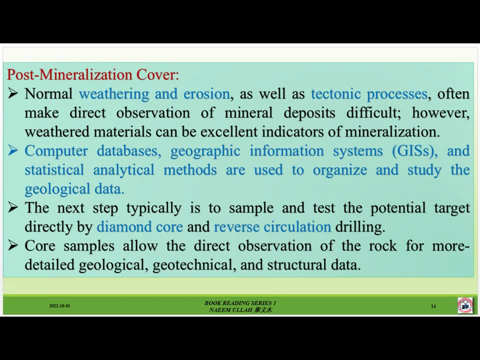 run wall cross境 marketипse Crossing space area. evely of the Three Electric teaches urban space war. in that exploration document all occurs from the stranger on work and temporal means. arrangement of events in time is called the temporal normal. weathering and erosion, as well as tectonic processes often make direct